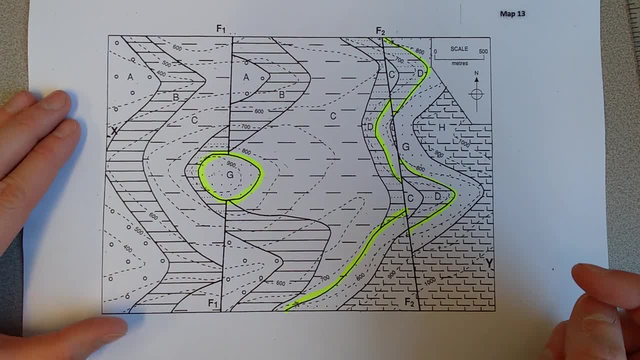 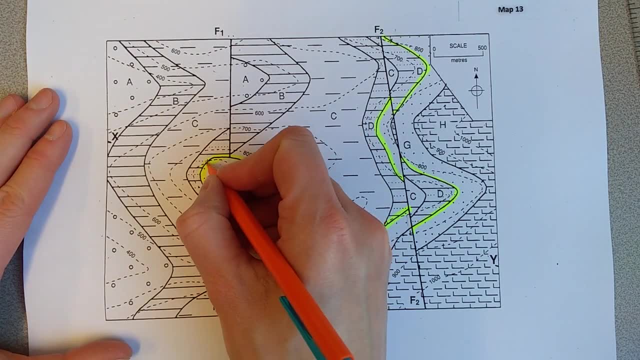 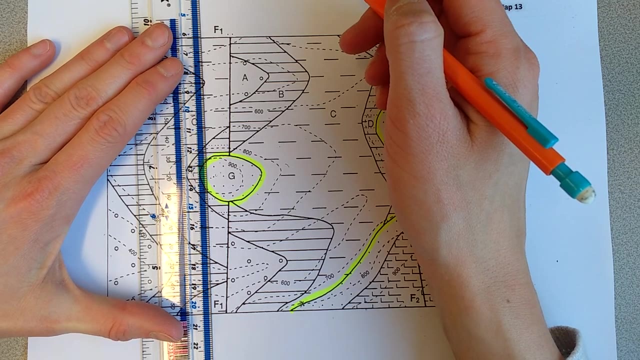 of our area for our unconformity. So remember to draw our structure contours. we need to identify points of equal elevation So you can see for this isolated part of my unconformity. it crosses through 900 and 900 of my topographic contours, So I can draw my structure contours. 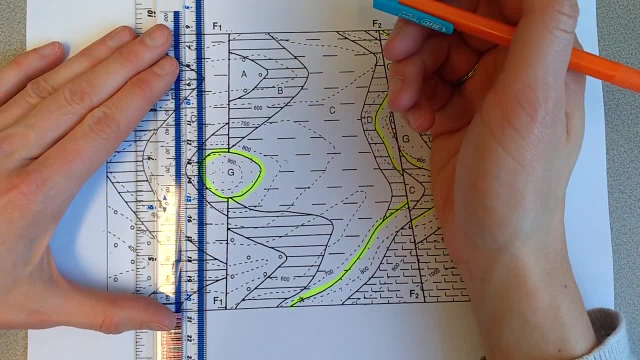 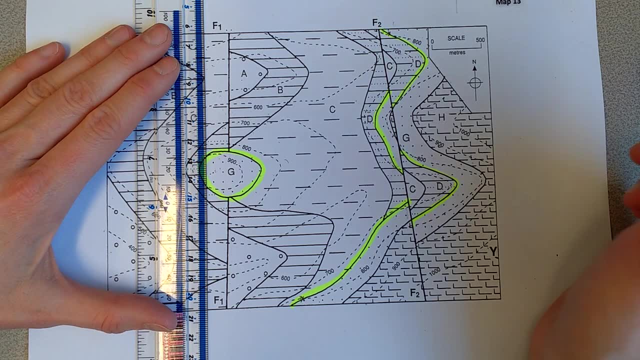 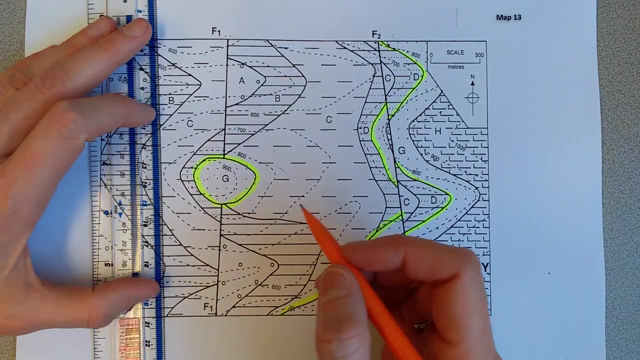 through those points Now, because these two intercepts are quite close together, it's a bit challenging to know exactly what the orientation of my line is going to be, And so ideally you want to also look at areas where you've got further apart intercept points. So I'm just 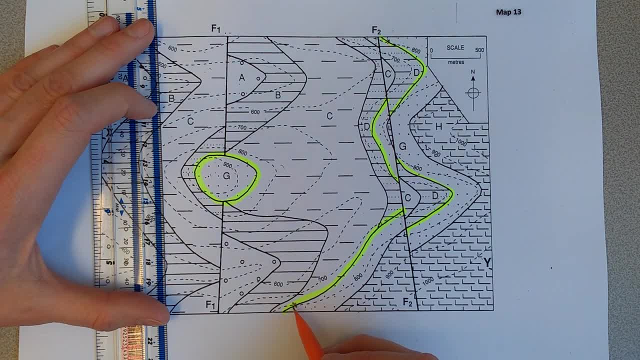 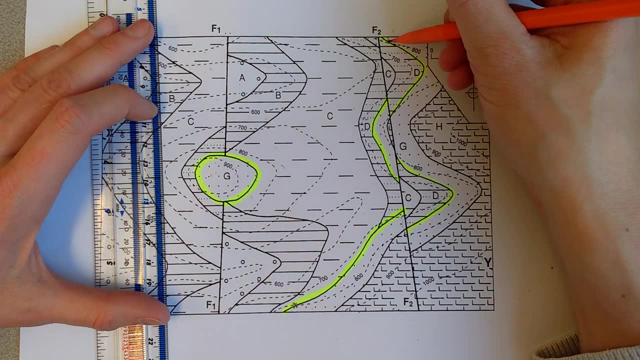 going to draw one example, because I don't think you've seen this area before. I'll go over that. And the two intercept points are quite close together. So I have this shared section of this column above and then I have an other intersect point on the other side. 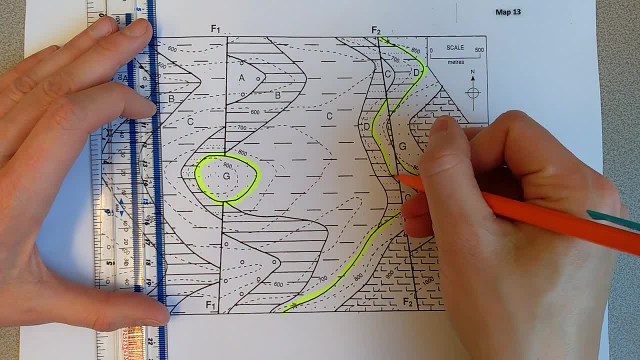 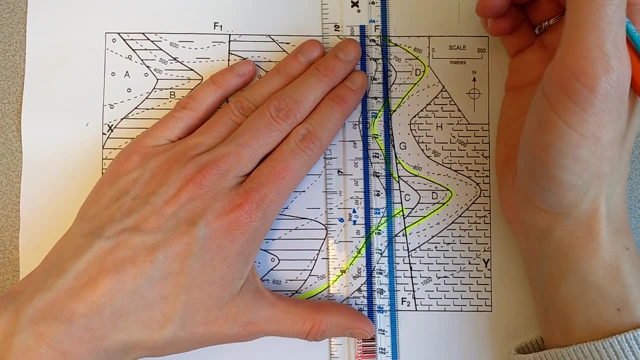 of it So I can observe these two intercept points on these other parts of the tractor, And then I can use my general obligations to inspect the intersection And as split nodes are flakes of water on the top of the bdena structure over it, I can then also locate. 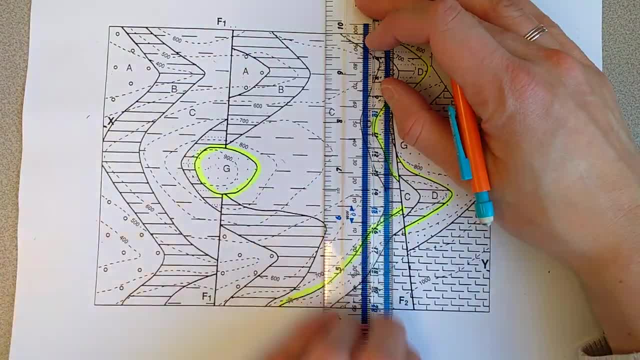 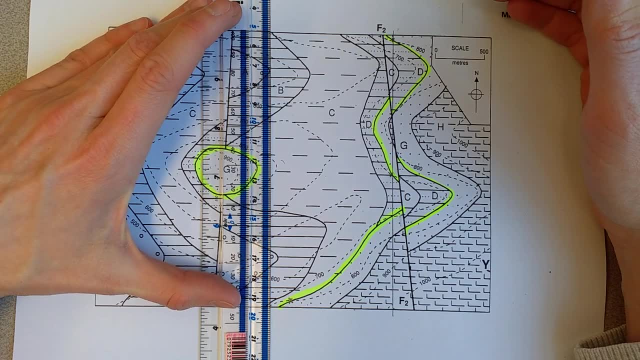 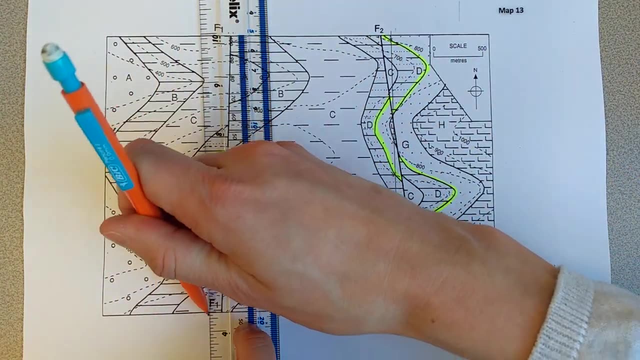 that big cluster bolt in the middle right corner over this section. This is where we're going to place these intercept points on the top right. define the geometry, then what I want to do is draw ones which are parallel across the map. okay, so you see that my ones through my two 800, 900 meter points through g. 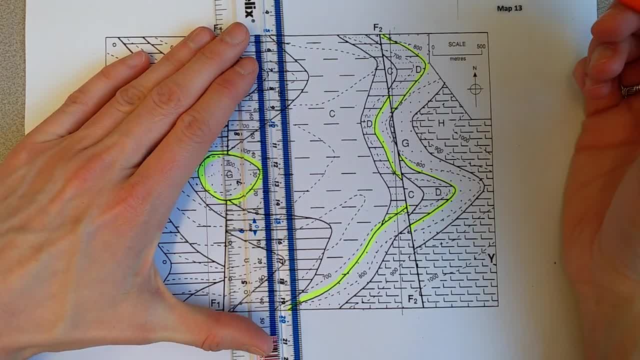 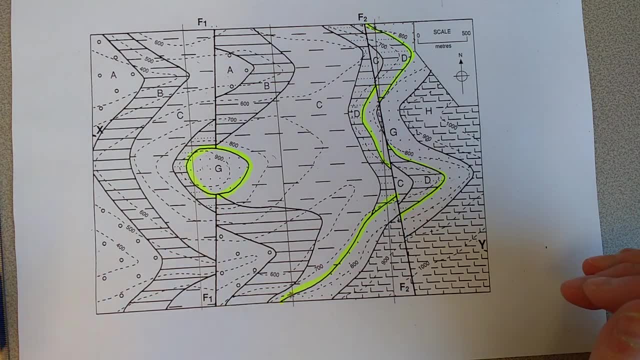 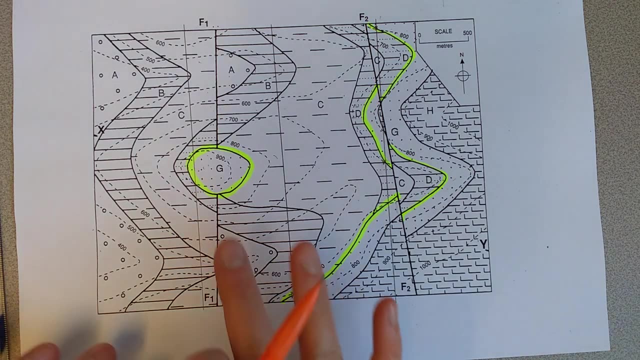 the unconformity there, and then I've got ones that go 800 there. so I can draw three structure contours. now they're not completely evenly spaced, don't think, but hopefully they're at least roughly. so what I'm going to do is label these now. so I'm going to do this systematically. 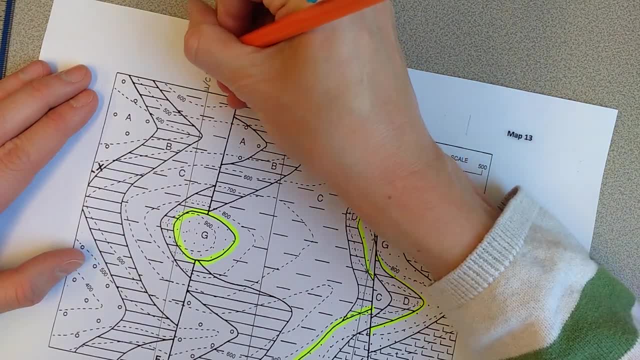 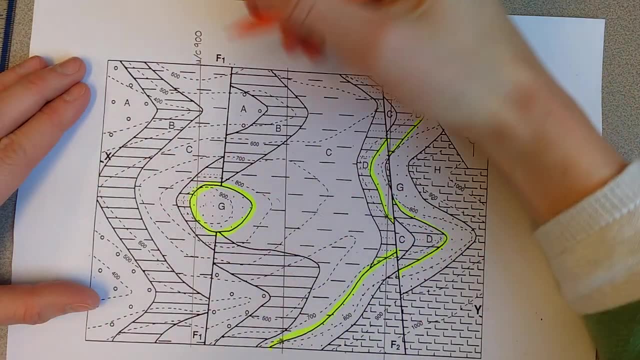 so I'm going to use UC for unconformity 900. now my numbers, I know I can predict are going to get lower towards the east of the map because my surface is dipping to the east. so this is going to be unconformity 800. 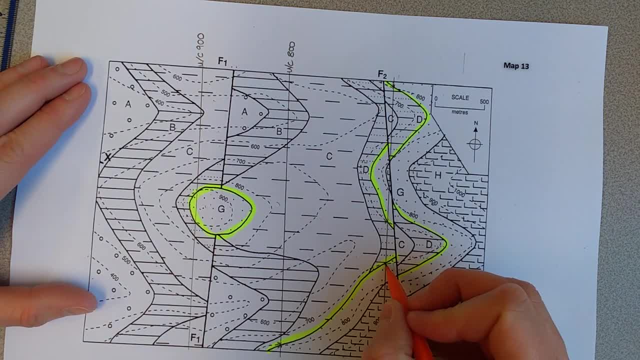 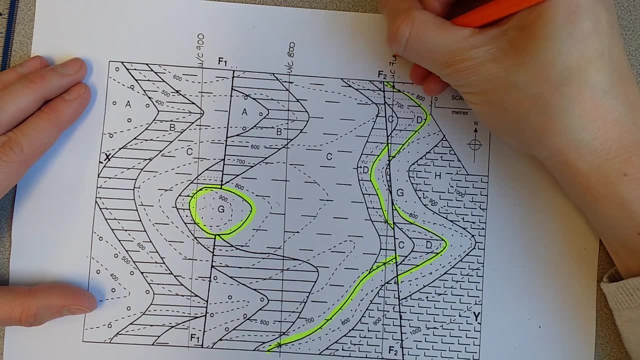 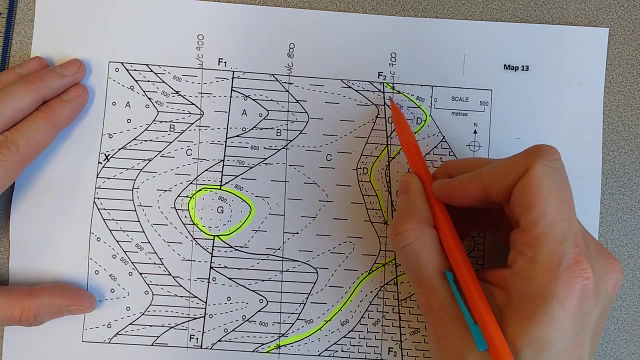 and then remember this one goes through my unconformity at these two intercepts here, which are 700. however, you'll also note that if we now go to the east side of fault two, that that is an 800 intercept point. so I can do two structure contours, two labels. 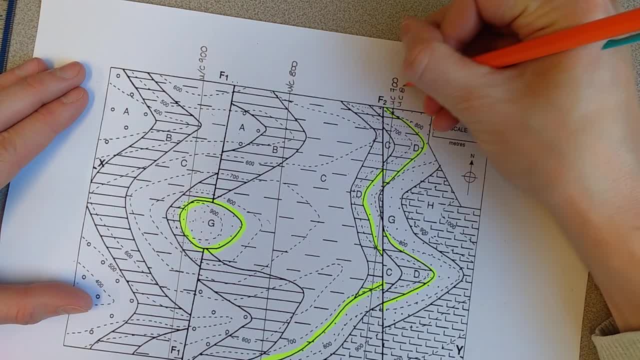 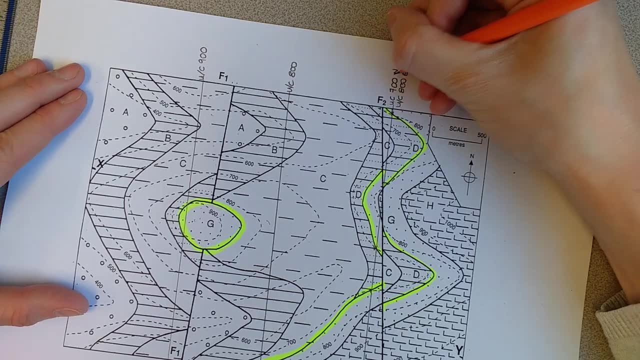 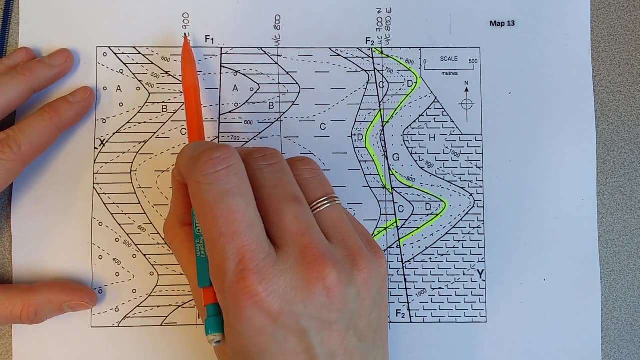 for this one structure contour either side of the fault. so it's going to be 700 to the west side of the fault and 800 to the east side, and that shows that we've got a 100 meter offset on fault 2.. so I've drawn my three structure contours which I've labeled for the unconformity. 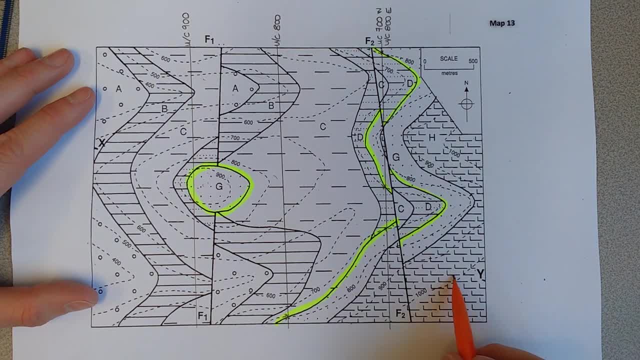 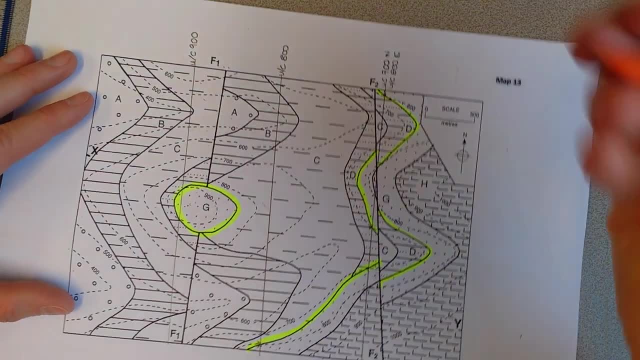 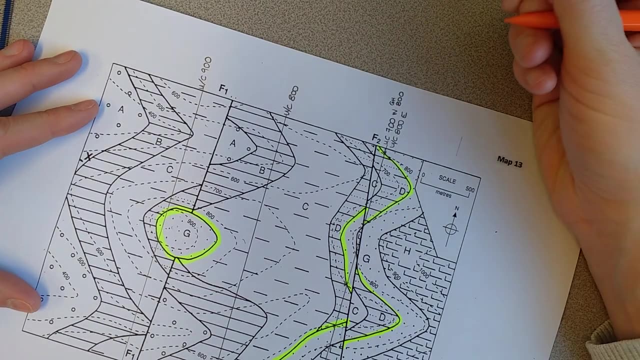 now you'll also note that we have this unit h, which is this brick pattern, and you can see here that there's an intercept at 800 meters for h on this one. so I'm going to add another label. so for my gh boundary is at 800 metres Now, as we know that these are going to systematically increase towards the west. 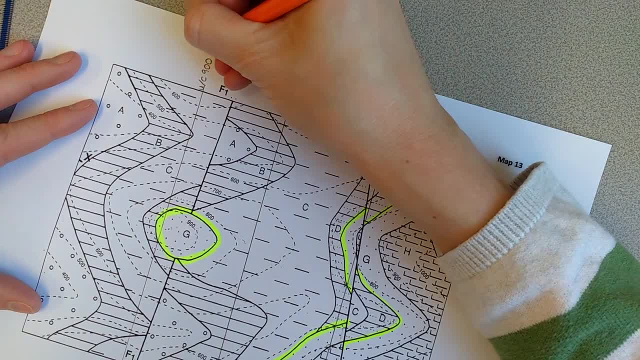 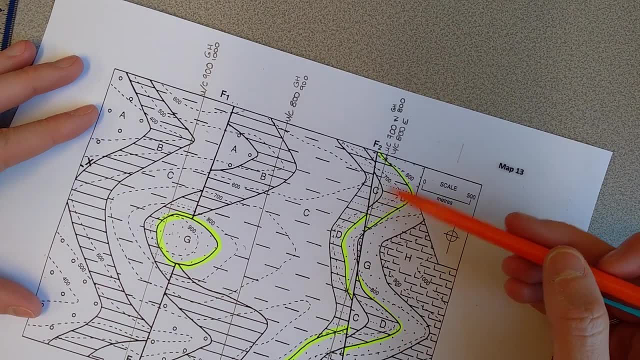 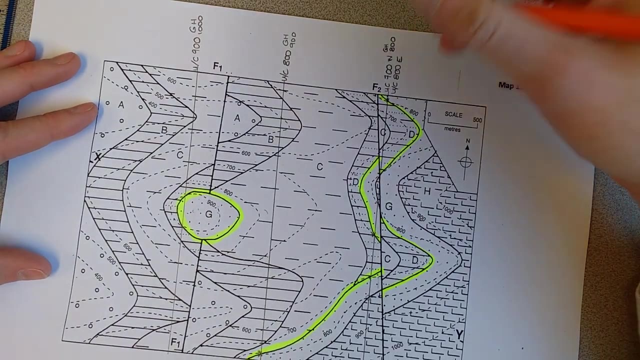 this would make this GH900 and GH1000.. So, and you can see, for this line we don't have an intercept point, but we know that we're going to have a 100 metre offset on our GH boundary as well, So that is going to be 900 metres to the east side of the fault. 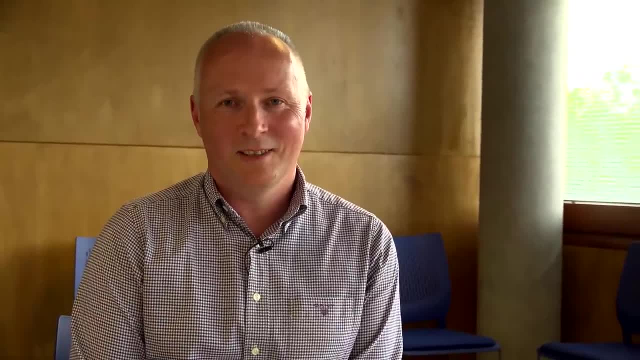 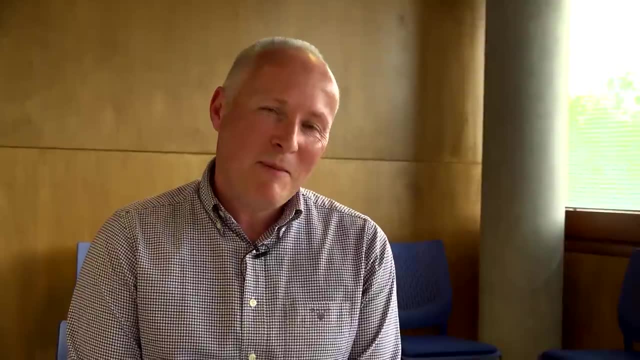 So we're doing this series, then, Graham, and thank you for coming back to Computerphile- about the most important thing in computing, or one of the most important things. Have you got something for us? Yeah, I think so. So maybe it's not the most important, but it's certainly one of.